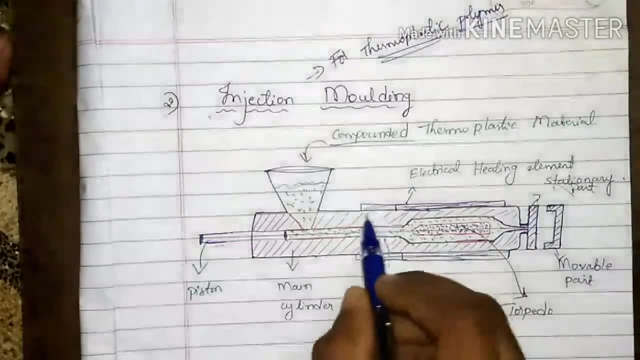 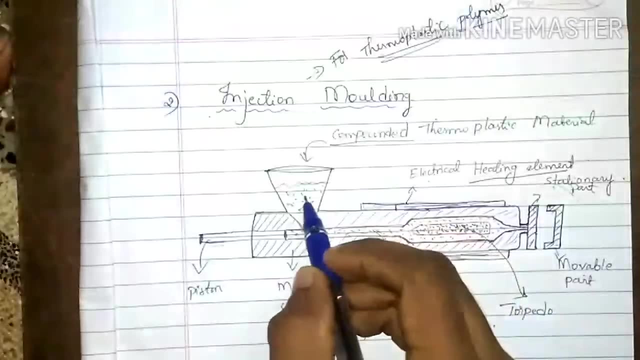 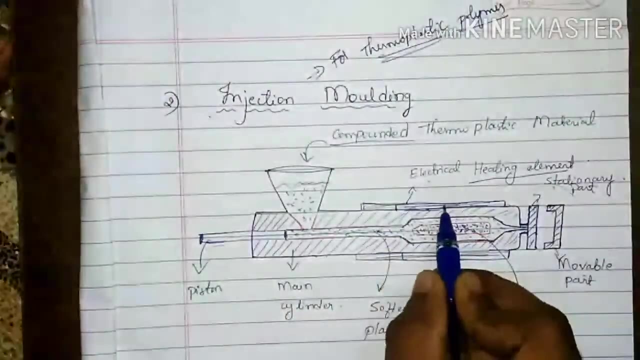 thermoplastic material further. okay, this is the cylinder and here you have heating element. okay, it is electrical heating element. okay, when the component thermoplastic material, which is in the powder form, and whenever it moves to this part, okay, where you have this heating element, that. 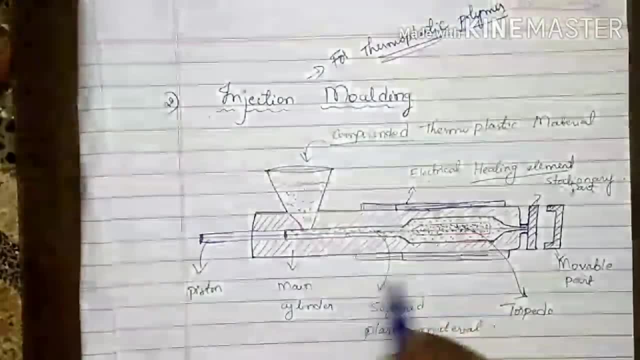 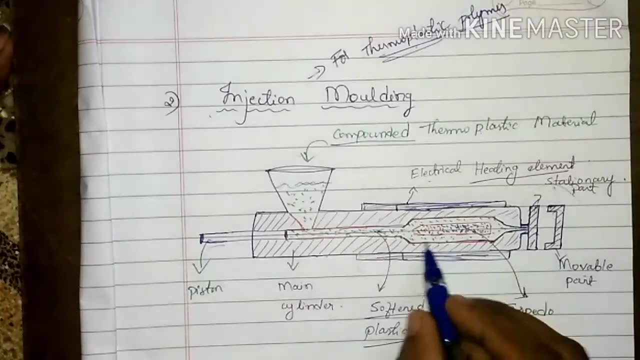 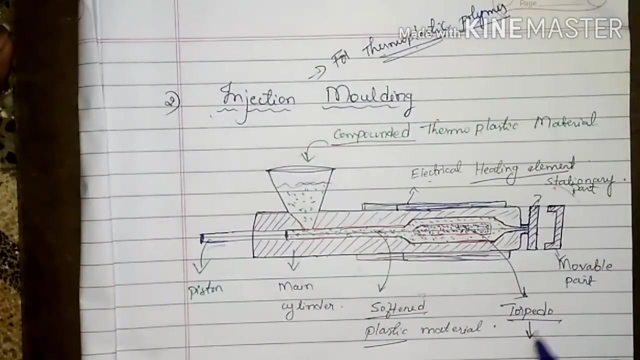 thermoplastic material met okay, here in this area. what happens? the powdered form of the polymer will melt, okay. it will get softened, okay. and here you have another part. now here you can see one part over here. that part is a torpedo, okay. torpedo means it is the part that is used to give the uniform heat distribution, okay. 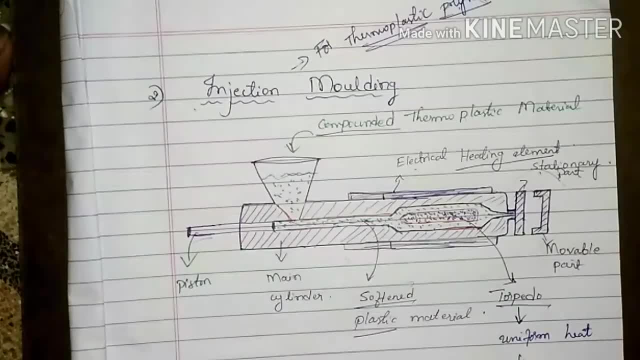 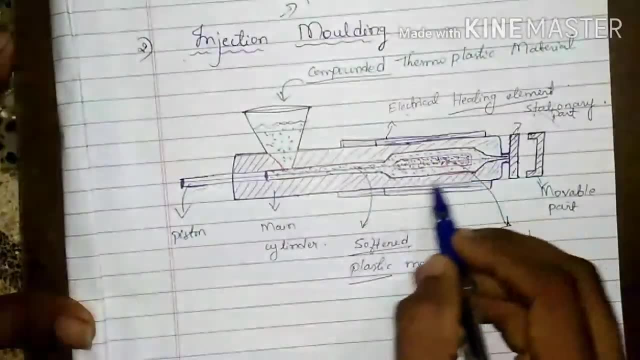 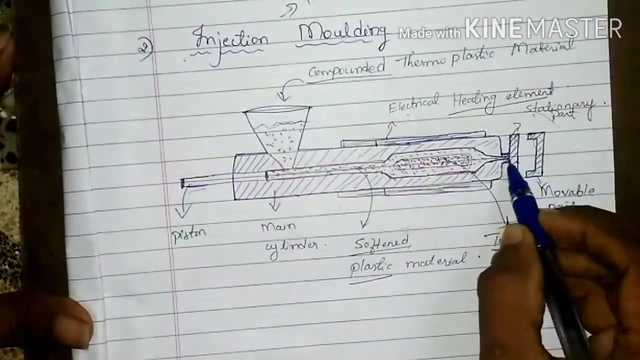 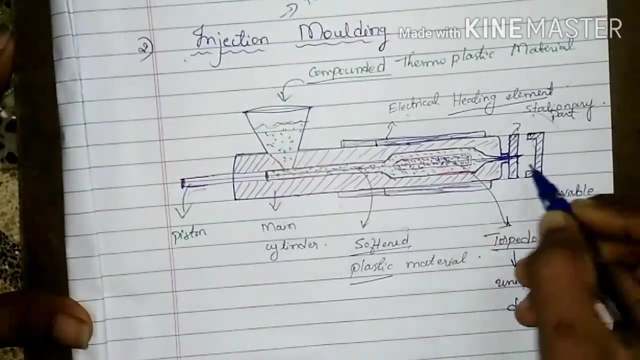 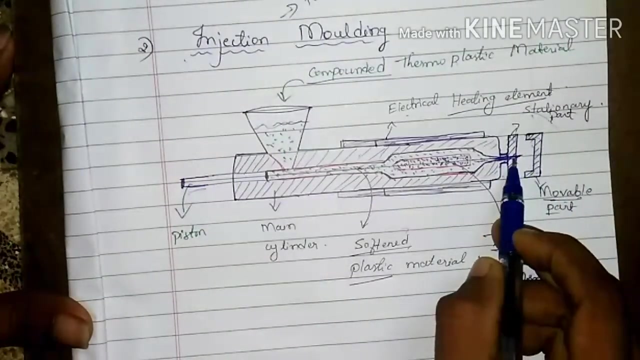 it is used to get uniform heat distribution. okay, here you have the molten form of the polymer and that is injected into here. okay, here you can see right. so this molten form of this thermoplastic material, it will be injected into this cavity. okay, and this is already. i said, this is a movable, so you have to close this mold onto the stationary. 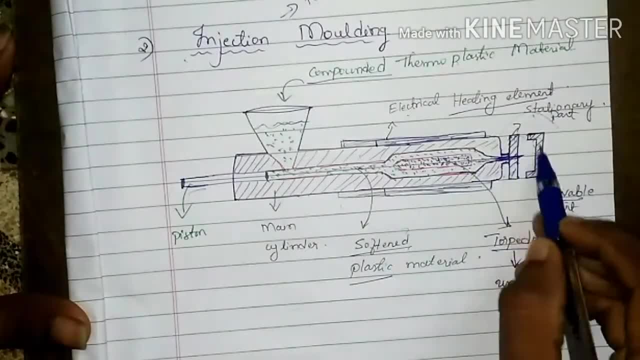 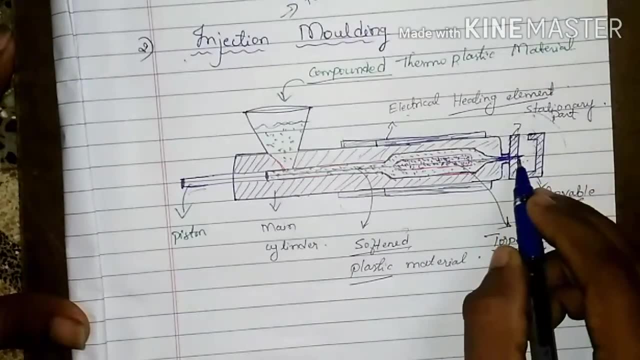 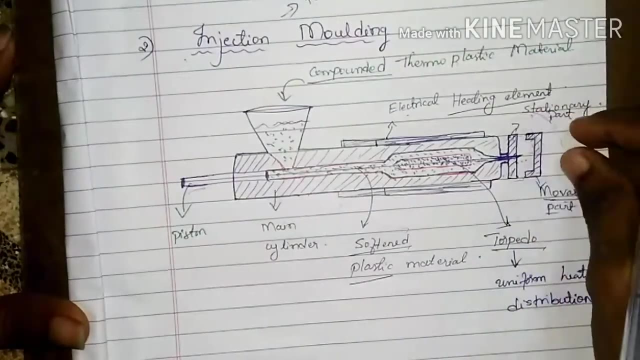 part and the once the more this polymer is injected to this mold. it is kept cold, okay. once the polymer melt is injected to this mold, what you have to do you just need to cool this mold. okay, once that part mold is cooled completely, then you open it and the- uh, you know the softer needle. 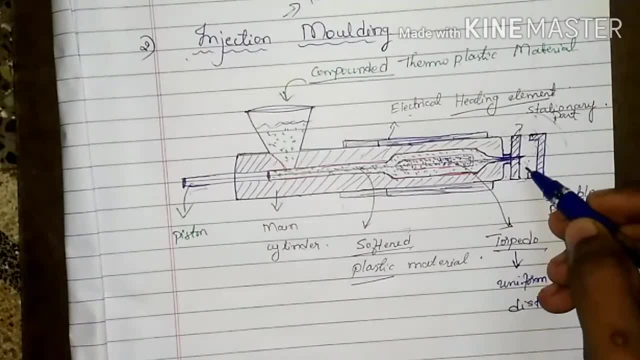 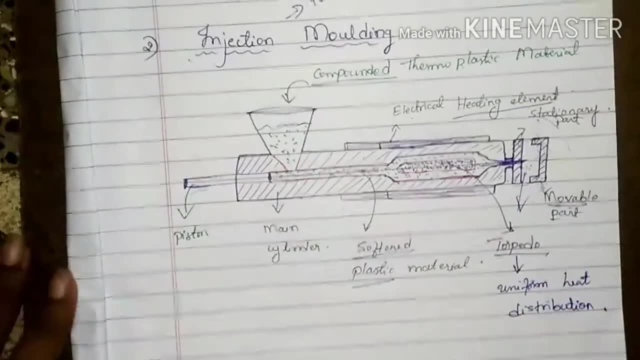 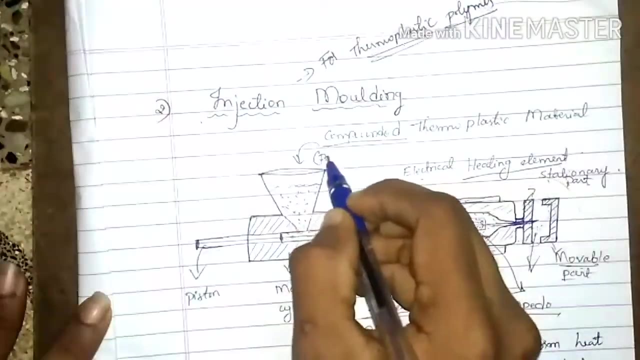 i'm sorry, the solidified uh uh uh article, the thermoplastic uh article. no, that will get ejected. okay, this is a very simple method, uh, that you can see in the injection molding. okay, first, what you need to do. first, you need to take the compounded thermoplastic material which will be in the powder. 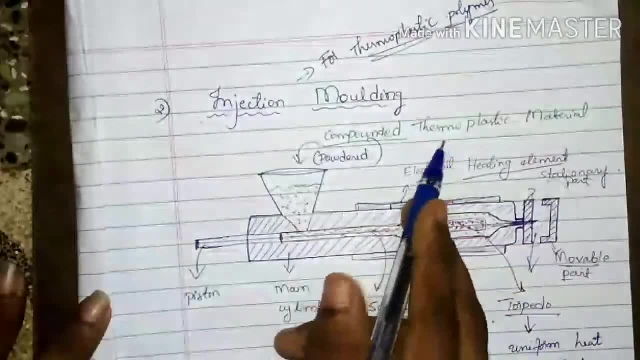 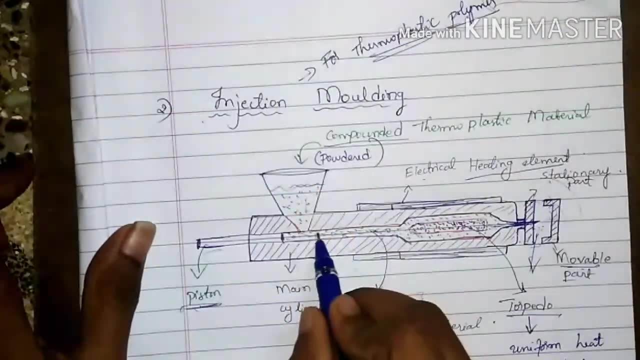 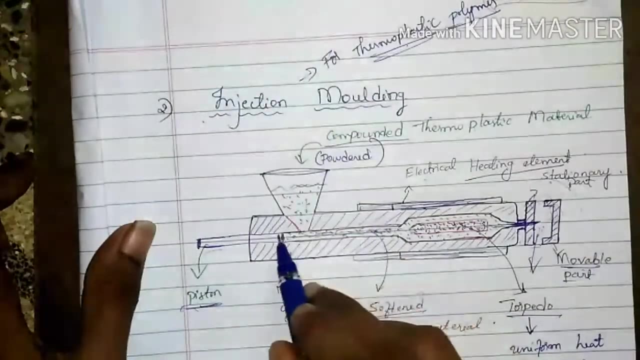 okay, and that powdered form of thermoplastic material is pushed forward by board, by the piston. okay, it can be moved like this. okay, you need to push it like this so the powdered form of that polymer will move here in this cylinder. then, whenever the thermoplastic material come to this region, what happened? it will get. 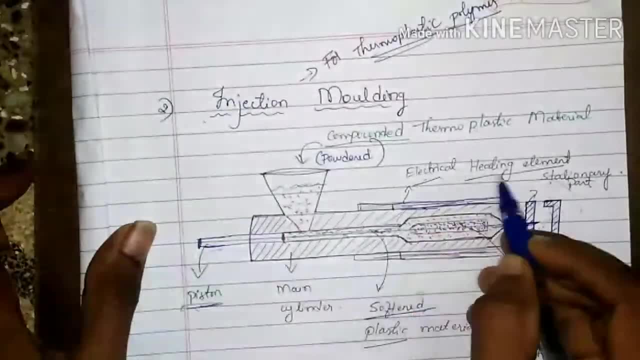 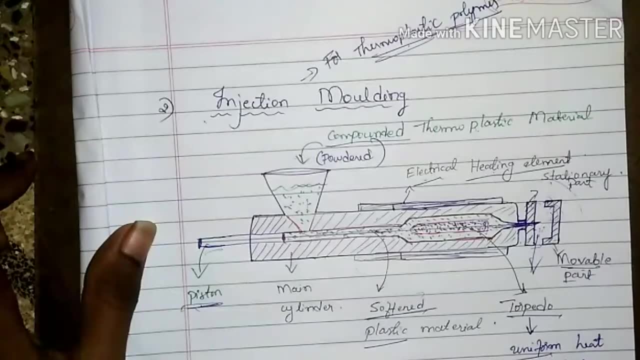 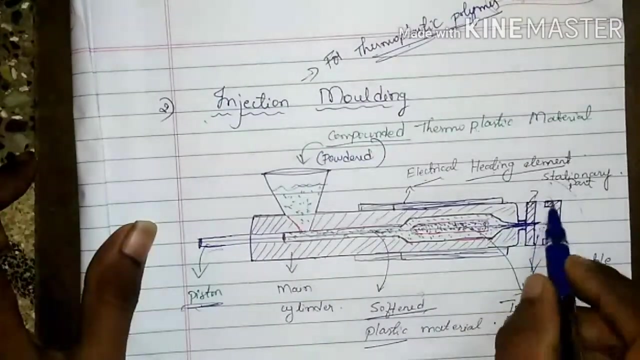 softened. okay, why? it is because here you have electrical heating element, okay, and also you have the stir pedal and torpedo will give us what uniform heat distribution that is mainly used heat distribution, and the, the softened polymer material is injected into this cavity and you need to close it. okay, initially you need to close it and you, then you have to inject it. then 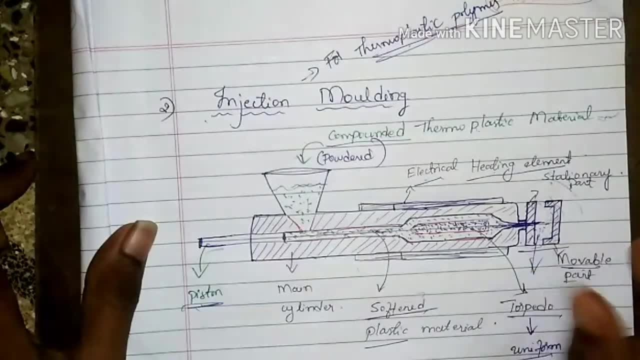 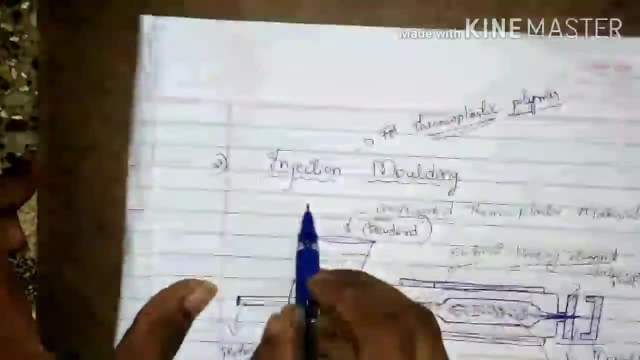 what you need to do. you just need to cool it and once it is cooled completely, just open it so that the polymer article get ejected out. okay, this is a very simple method that you can see in injection molding. okay, if there is any doubt in this injection molding, uh, let me know. okay, and in the 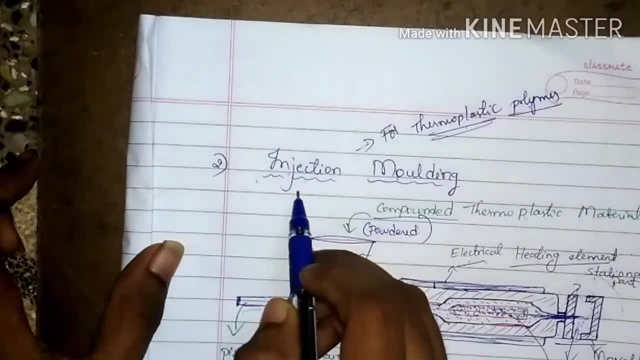 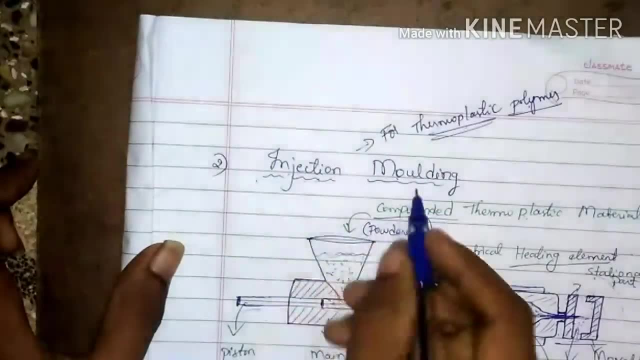 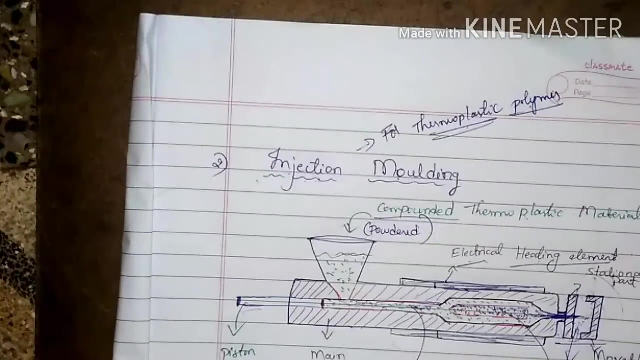 next video, we will talk about extrusion molding. okay, this is the injection molding and just similar to this injection molding. you have extrusion molding. okay, after that we will see blow molding. okay, by that the molding is done and then we will move forward to other polymer processing techniques. 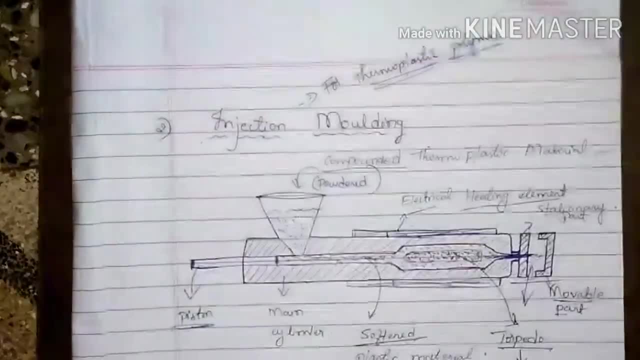 okay, thank you for watching. if you have any doubt in this video, please let me know okay. 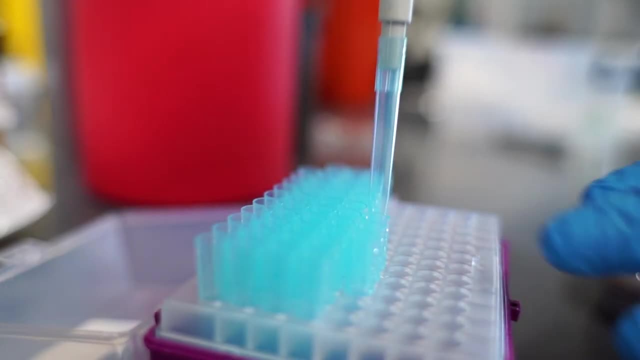 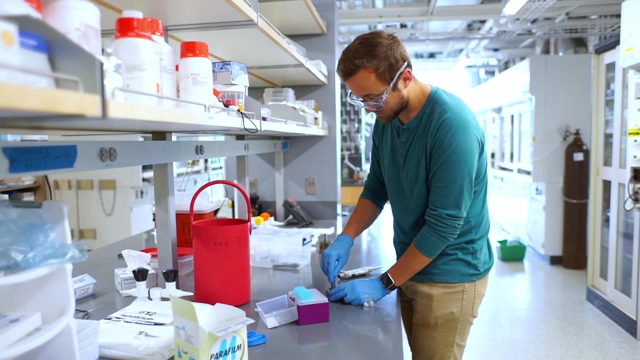 Code centering is a technology that was developed at Penn State around 2015 or so by the Clive Randall Group, And one of the things that we realized right away is that it's a great opportunity to be able to then make composites. 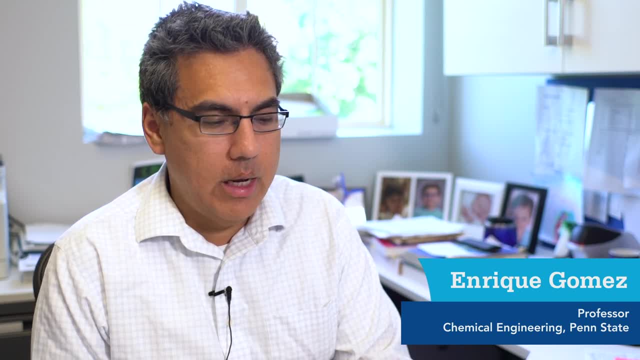 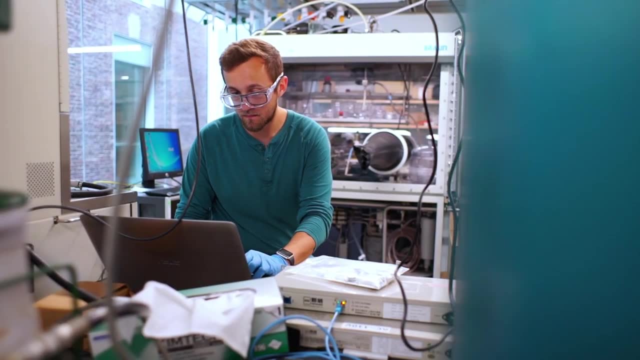 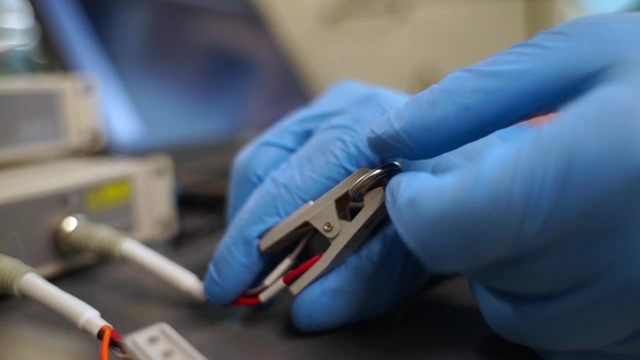 To basically merge organic and inorganic systems together in a way that hasn't been possible before. The key is to continue to demonstrate how end of life can be incorporated into the design process, Because the processing is so straightforward, so green. if you will, that means that we can do it over and over again. 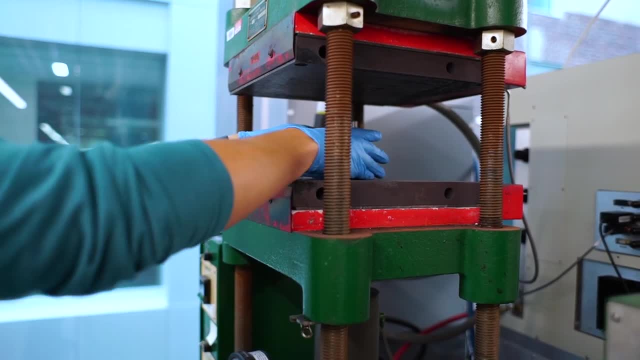 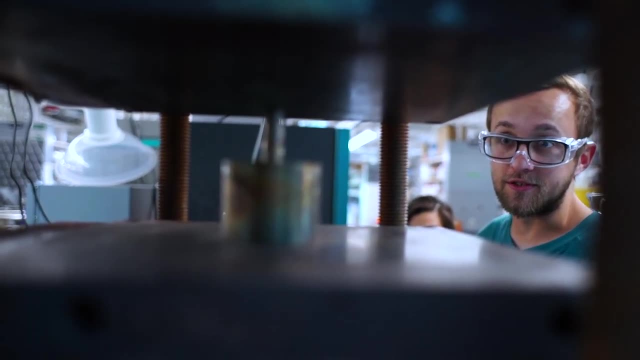 We're going to be able to take this technology and we're going to be able to demonstrate its impact, Not only in making different types of materials that have unique functionalities, unique properties or something like that, But also types of materials that will eventually lead to reduced waste.